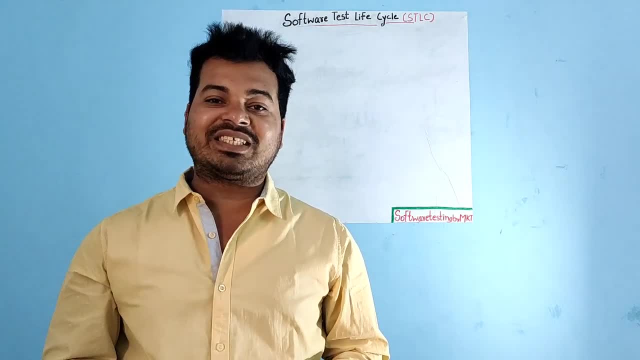 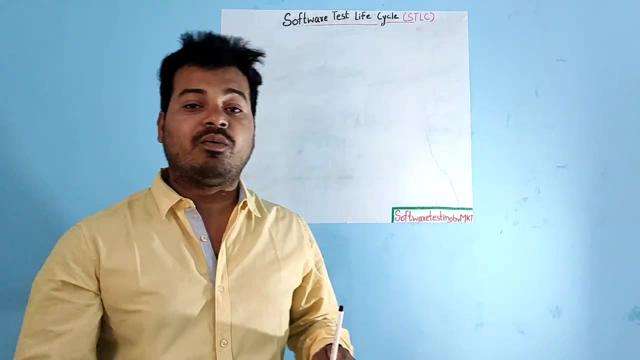 Hello everyone, I welcome you all to my YouTube channel, Software Testing by MKD. In this video, we are going to talk about a very important topic in software testing which is called as. what do you mean by STLC? also called as Software Test Life Cycle. So let's get started. 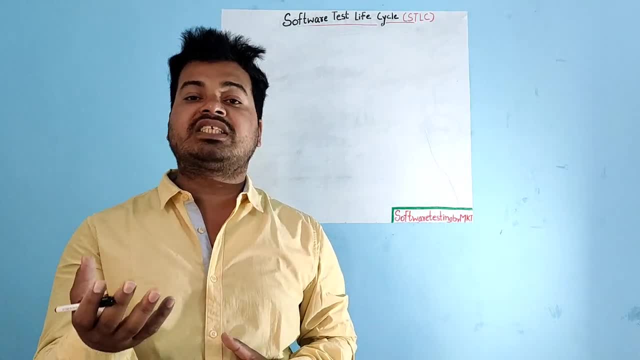 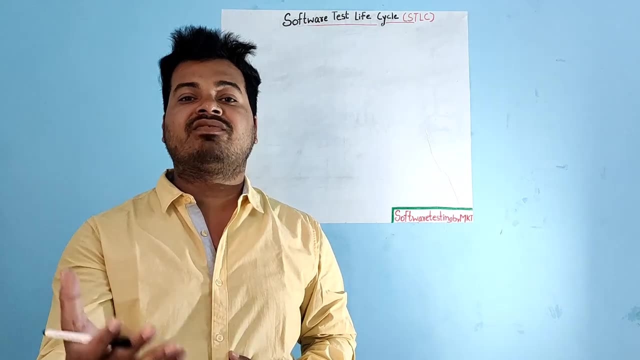 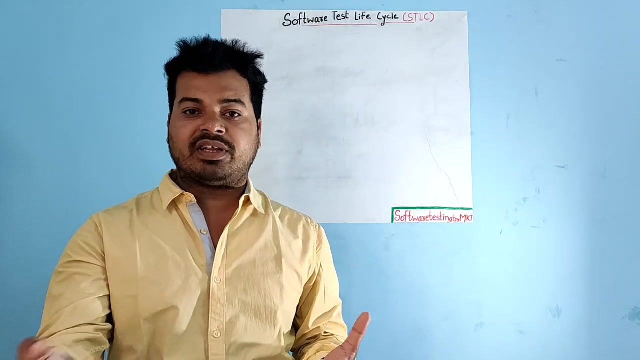 So STLC. it is a step-by-step procedure or a standard procedure to test any new software. That is called as Software Test Life Cycle. It is a step-by-step procedure or a standard procedure to test any new software That is called as STLC. 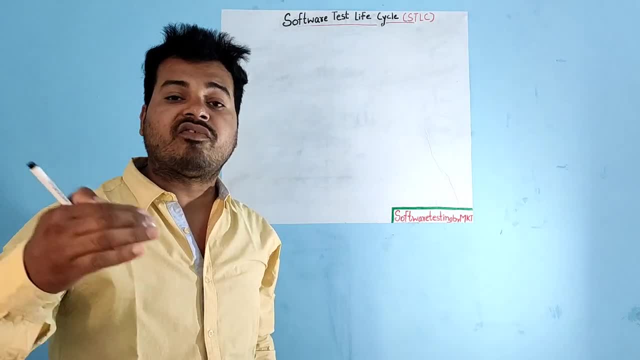 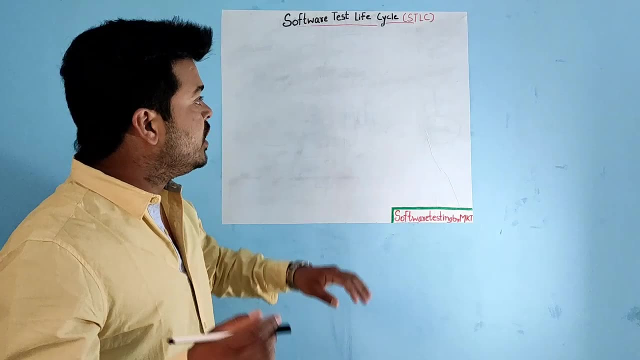 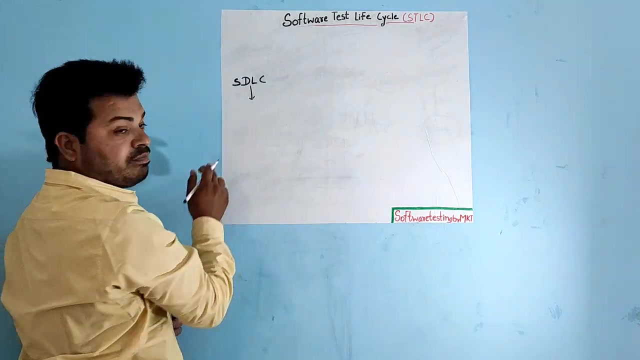 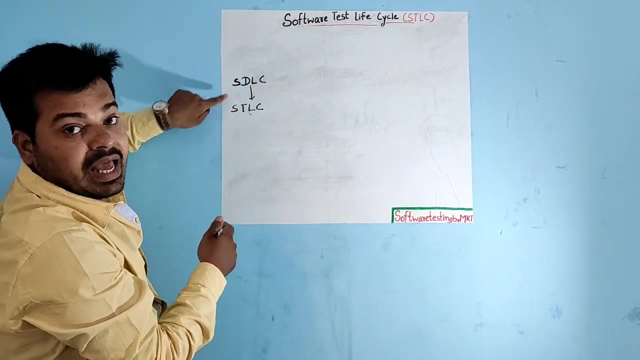 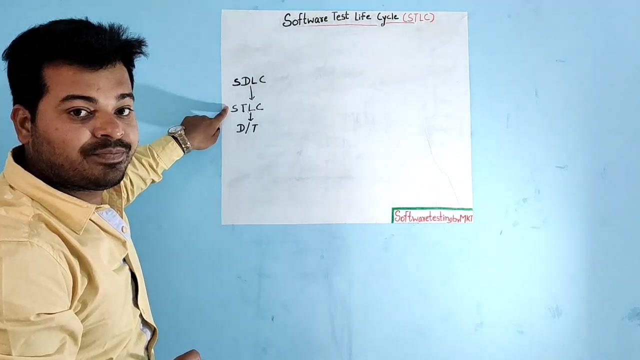 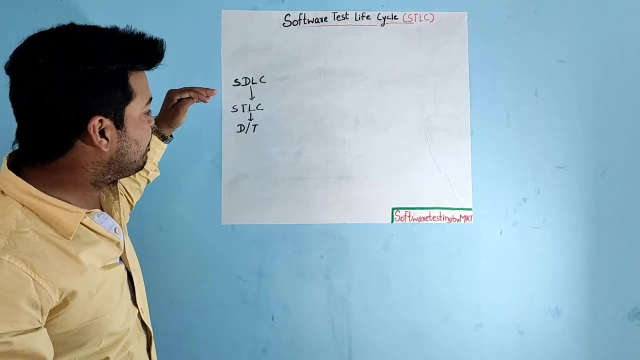 Now, if you guys remember my STLC video- Software Development Life Cycle video- if you don't remember anything, link is there in the description. Please check it out. Please check it out and please come to this video. So, if you remember my STLC video, so this STLC is a part of my STLC. My STLC is a part of STLC and my defect tracking- my defect tracking- is a part of my STLC, So my defect tracking, life cycle or bug life cycle, is a part of my Software Test Life Cycle and my STLC. 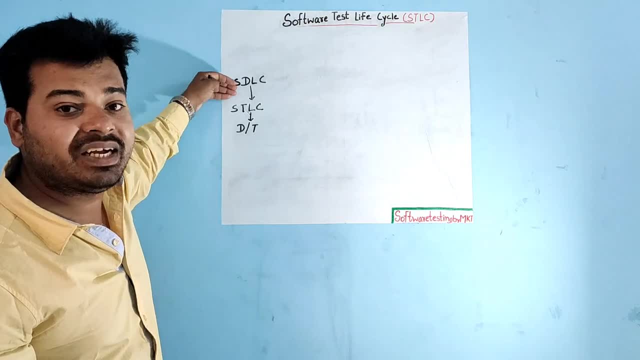 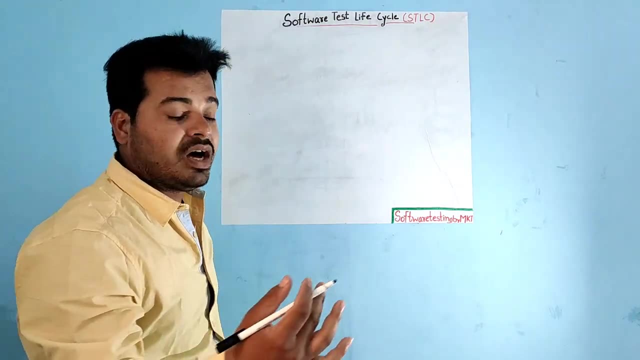 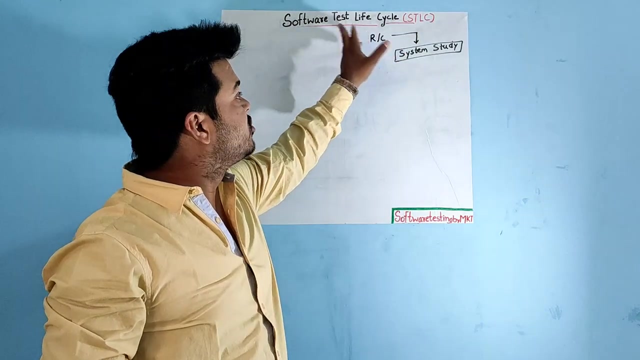 My Software Test Life Cycle is a part of my Software Development Life Cycle. Now, the various stages in my Software Test Life Cycle are Requirement, Collection and then System Study. This is my first stage of my Software Test Life Cycle, which is called as System Study. 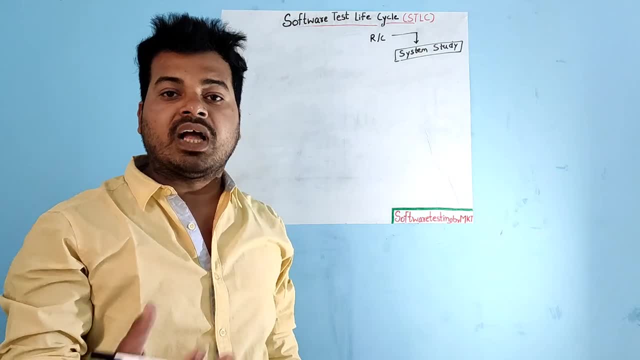 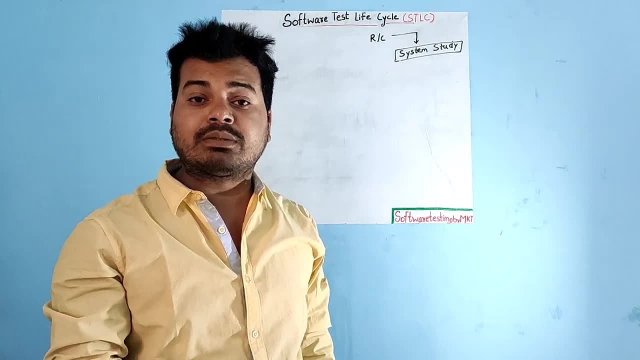 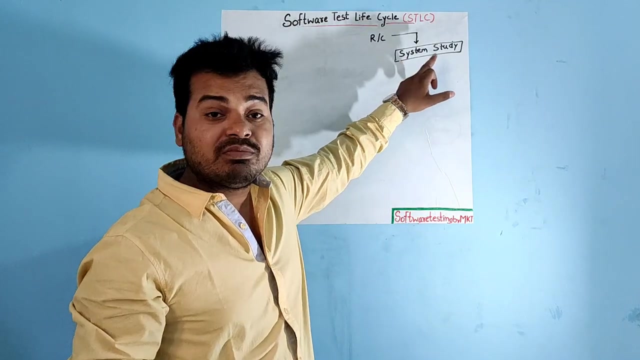 System Study is nothing but when customer gives the requirement, our company product manager will collect the requirement. come to our company, explain the requirement to our technical team, that is, both developer and test engineers. Making our technical team understand the requirement is nothing but System Study. 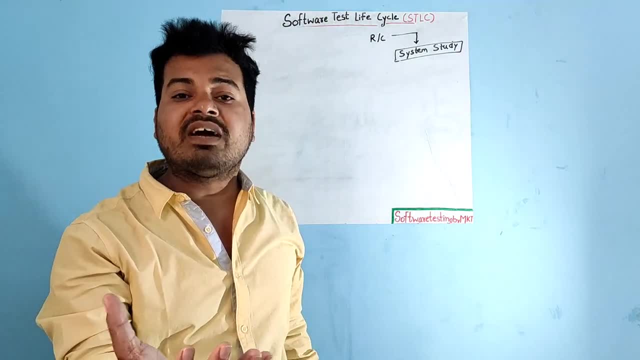 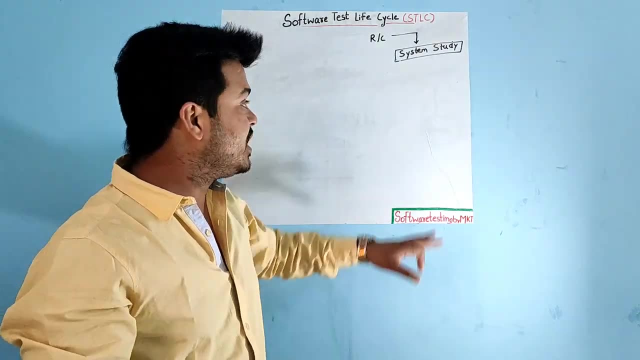 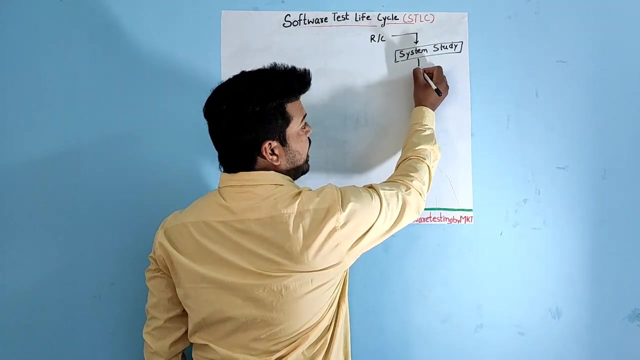 It is a study of the requirement to make our technical team, that is, developers and test engineers, making them thoroughly understand the requirement. It is nothing but System Study. And now my second stage of my STLC is nothing but Test Plan, Test Plan. 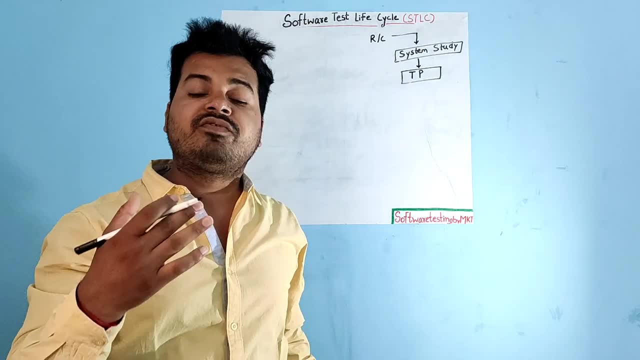 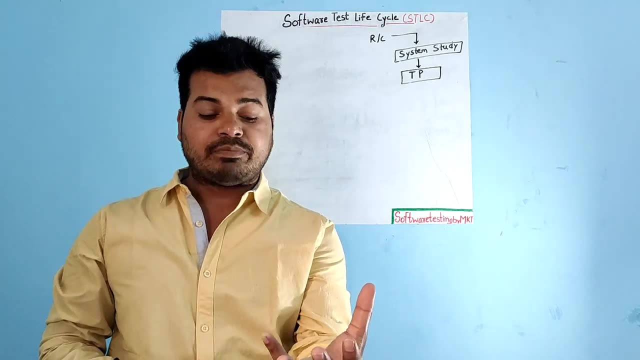 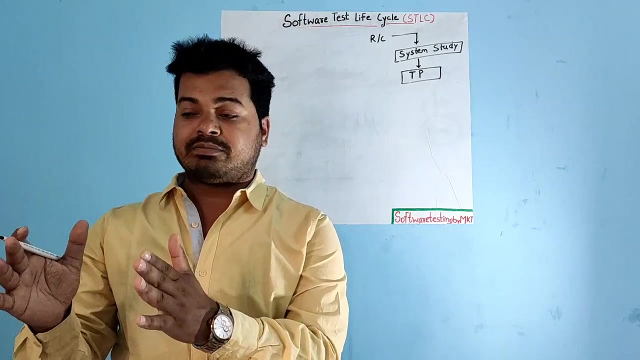 My Test Plan is nothing but all the future testing related activities. It is nothing but how many test engineers are going to work on this particular release, Which test engineers is going to work on which particular module, How many days my test engineers will take to complete this testing process for this particular release. 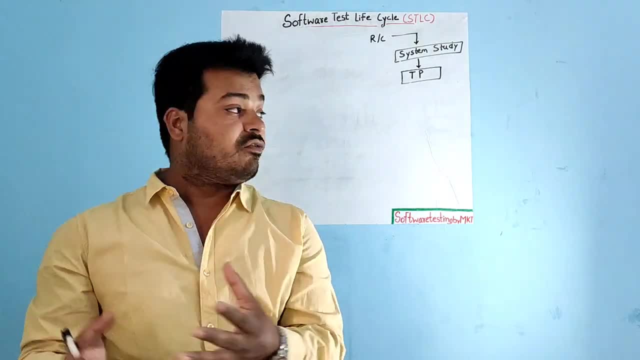 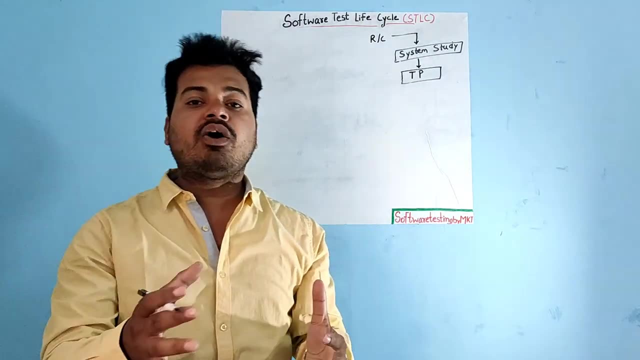 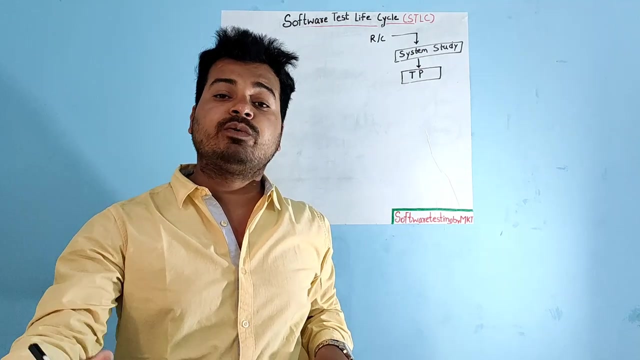 And which bug tracking tool which we are going to use for this particular release, Which automation tool We have to use for this particular release. So these are all things will be the part of Test Plan. It is a plan, It is a document which covers all future testing related activities. 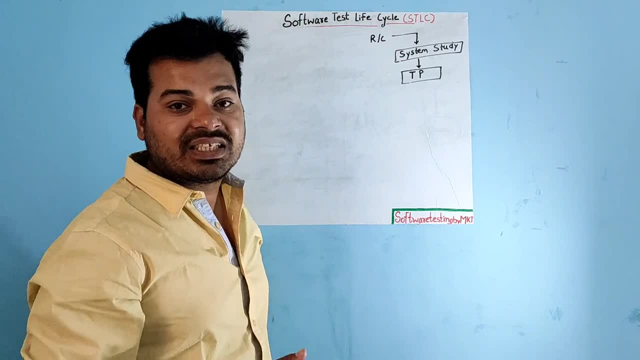 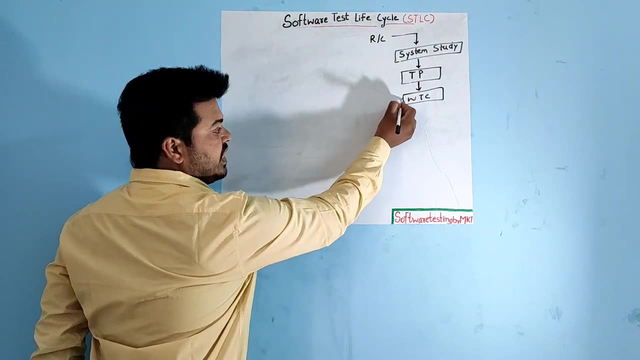 Now the third stage of my STLC is called as Write Test Cases. Under Write Test Cases, we are having multiple stages, which is called as System Study again. Now, what is the difference between this System Study and this System Study? Now, what is the difference between this System Study and this System Study? 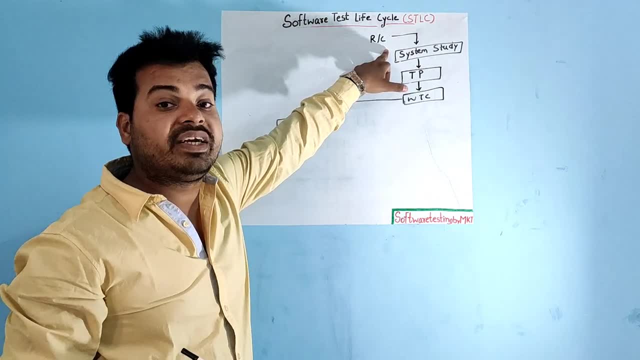 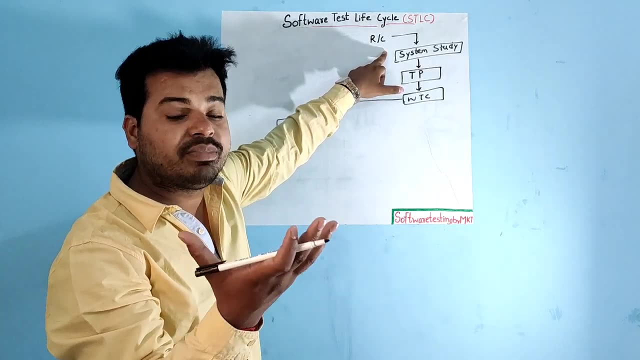 Now, what is the difference between this System Study and this System Study? This is the System Study which will be done by the BA Business Analyst or the Project Manager, Where he will give the complete knowledge of the product, Complete requirement knowledge he will give to the both developer and test engineers. 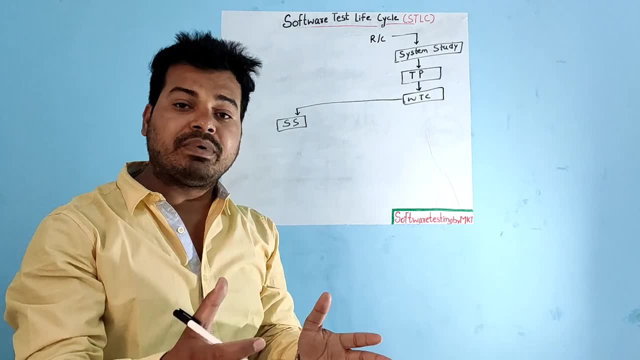 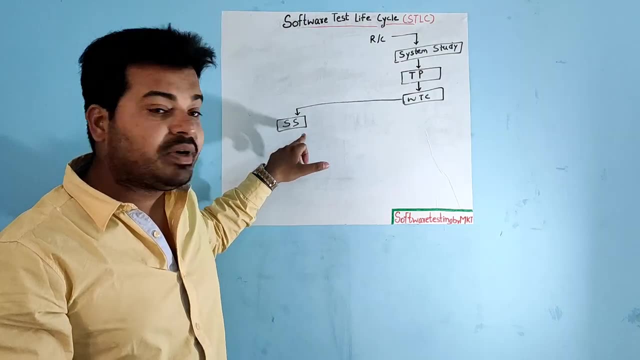 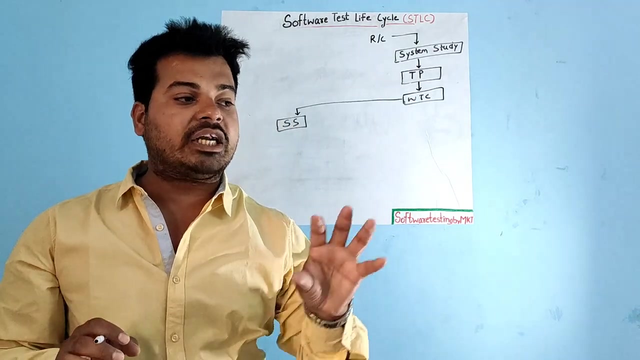 He will make all the technical team or all the people present in the company, understand what is the requirement Coming to this System Study? This is nothing, but it is a System Study which will be done by individual test engineers. Suppose there are 5 test engineers and each are assigned with a particular module. 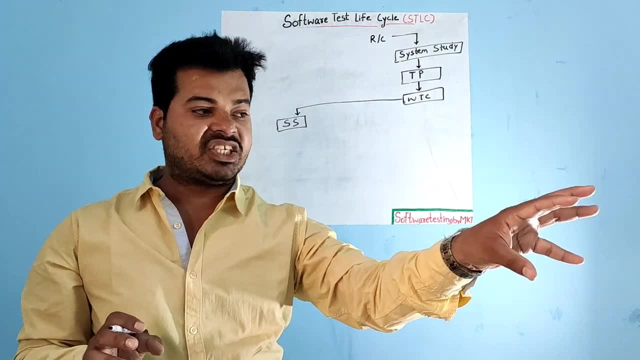 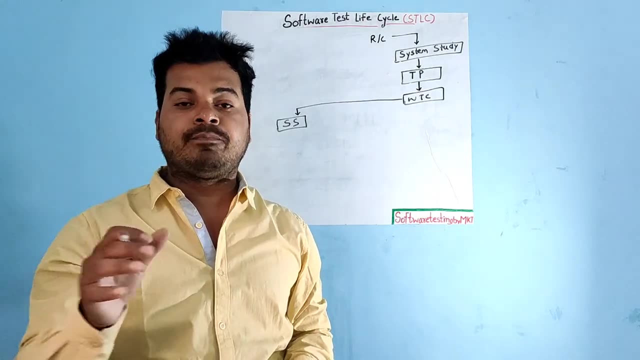 Like: A module is going to test by my this test engineer. B module is going to test by my this test engineers. C module is going to test by my this test engineers. So this System Study is nothing but each and every individual test engineer. 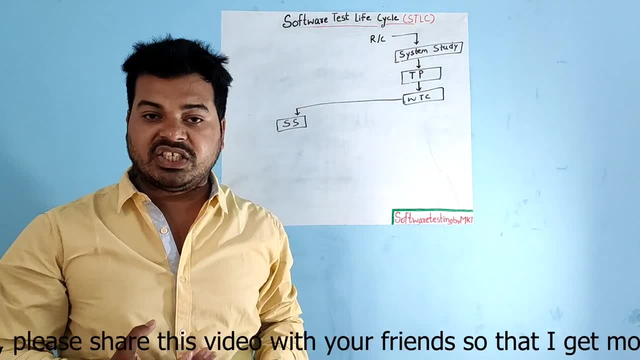 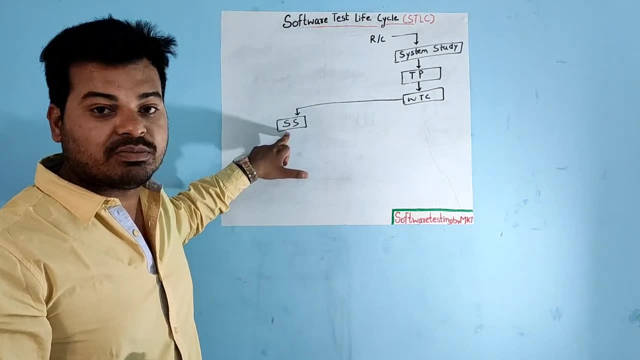 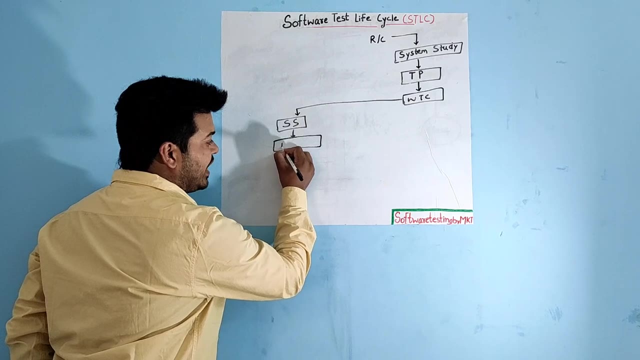 Whatever the module is assigned to that particular test engineer, He will study or he will try to understand that particular module in detail. That is called as System Study. Once after my System Study is done, We have to identify all possible scenarios. So identify possible scenarios. 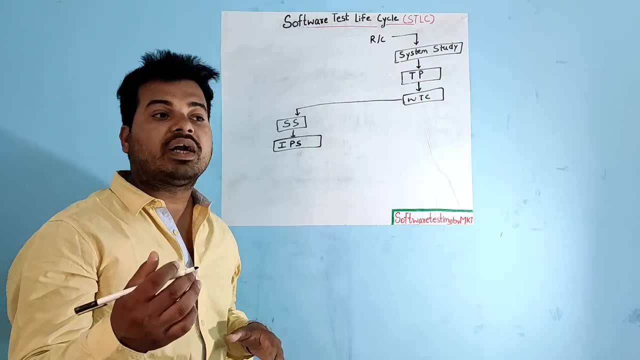 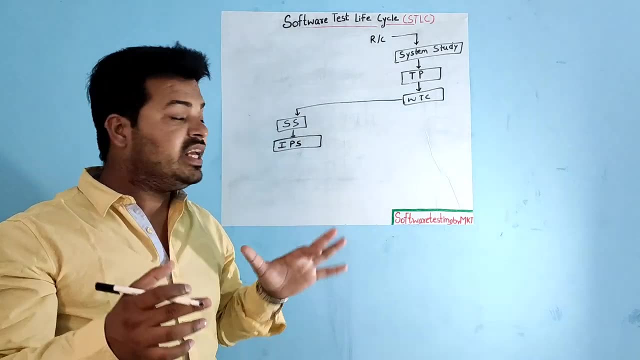 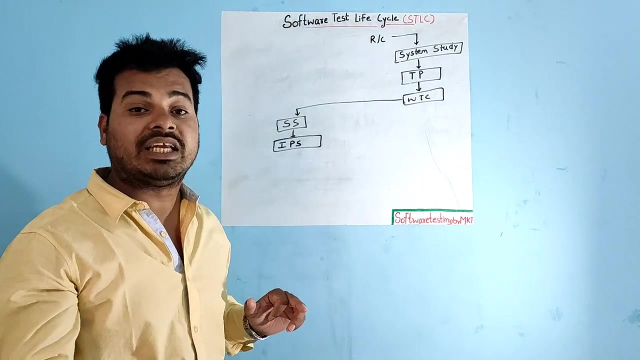 Identify all possible scenarios is nothing, but whatever scenarios I have to test my application, That scenarios we have to identify. Each and every individual test engineer will identify all possible scenarios to test the particular module which is assigned to him In this. the third stage is called. 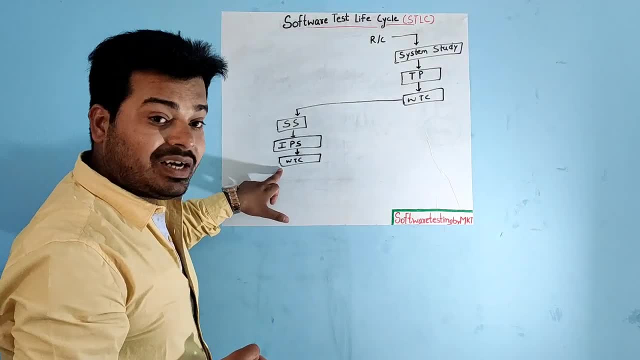 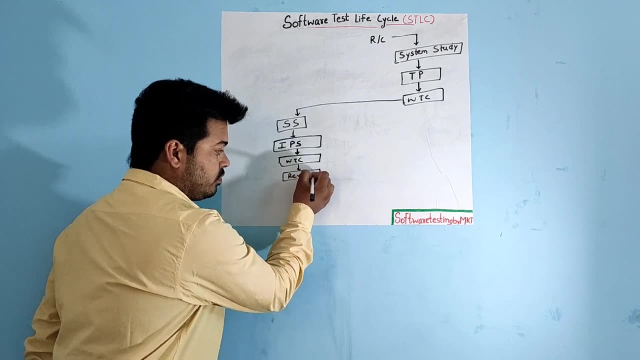 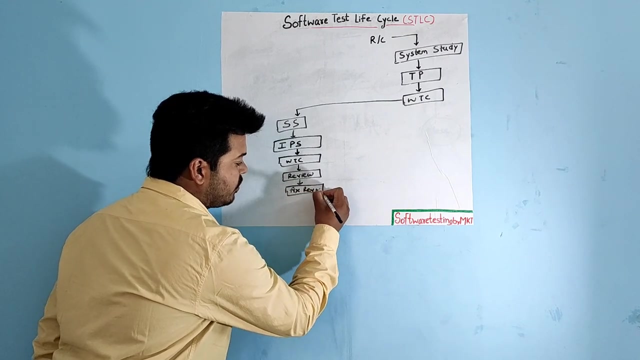 Write Test Cases Here. they will write all test cases. After writing test cases, they will make it review. They will get it review Once after review is done. We have to do Fix review comments. Fix review comments Once after fix review comments are done. 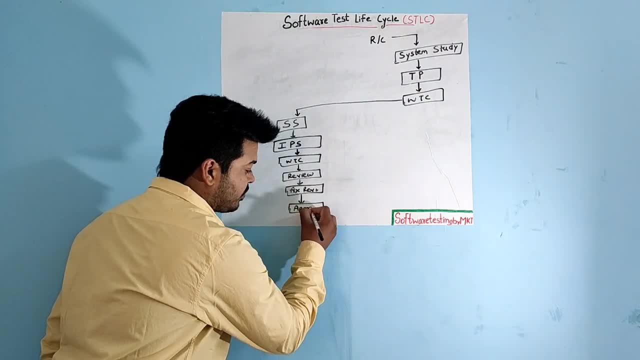 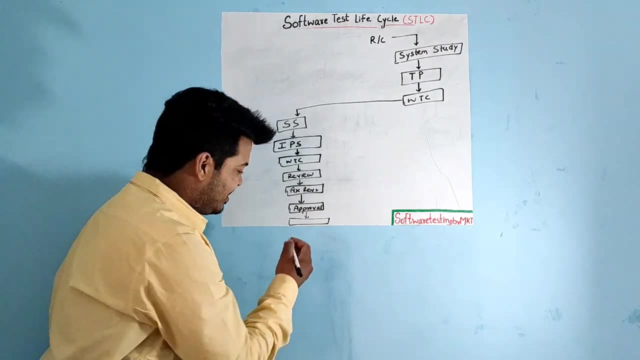 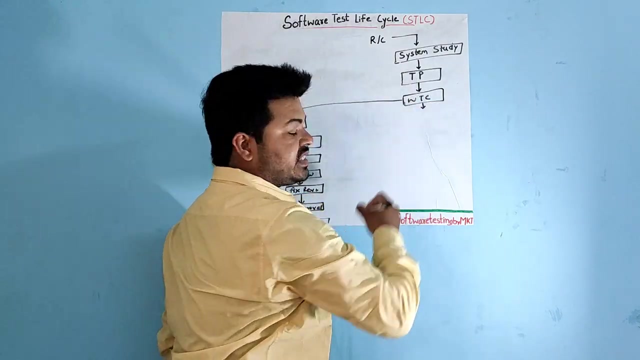 Then we have to get the approval. Once after approval is done, We have to store our test cases In test case repository tool. So under write test cases. These all are the stages. Now, once after my test case part is done, We have to write traceability matrix. 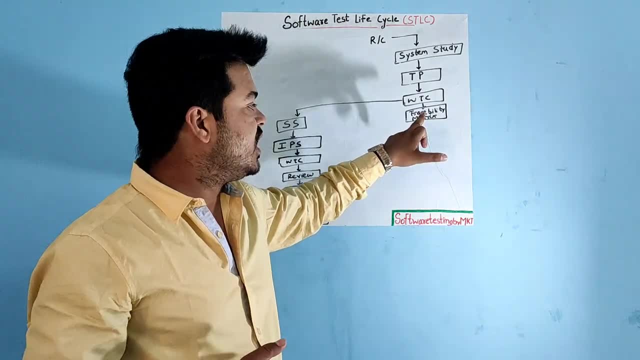 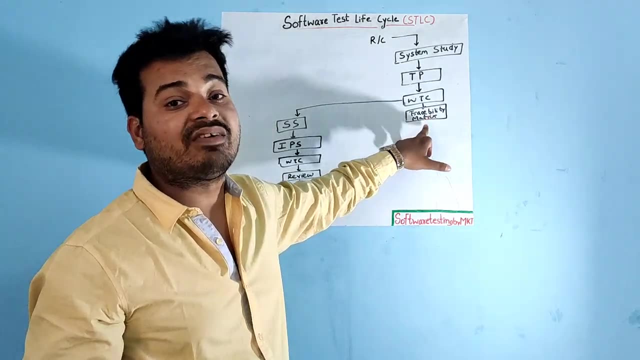 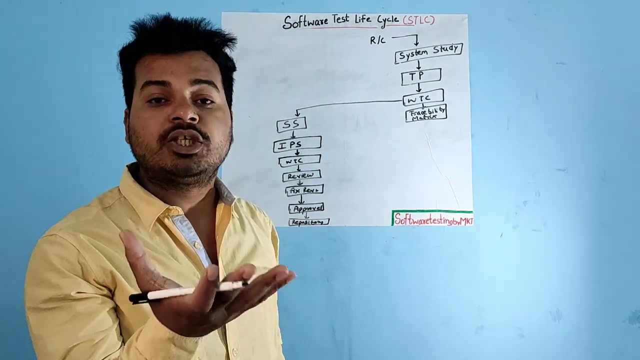 We have to prepare the traceability matrix. The other names of traceability matrix are also called as Requirement traceability matrix And also cross reference matrix. Now, what exactly is my traceability matrix? Traceability matrix is a document Which ensures that. 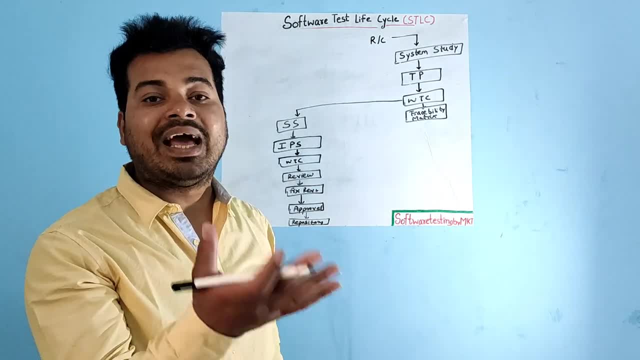 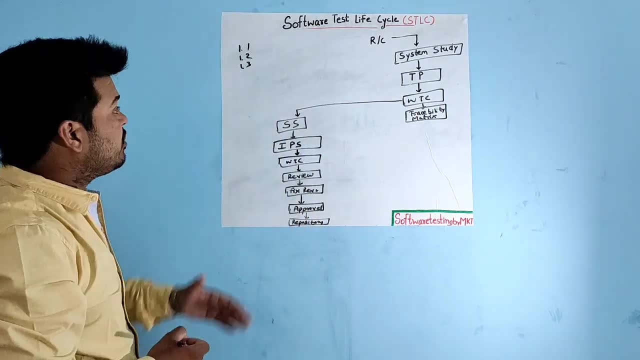 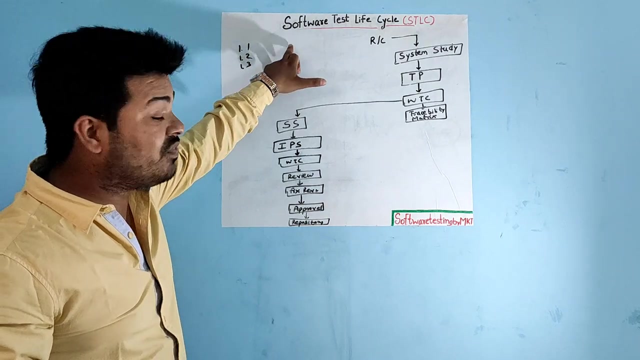 Each and every Requirement has got At least one test cases in it. When we are having the list of requirement, When we are having all the list of requirement, We have to make sure that Each and every requirement Has got at least one test cases in it. 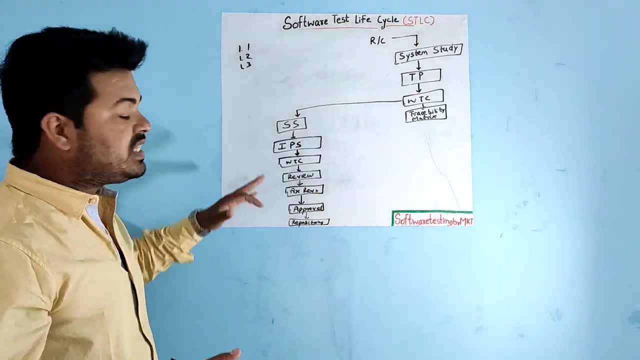 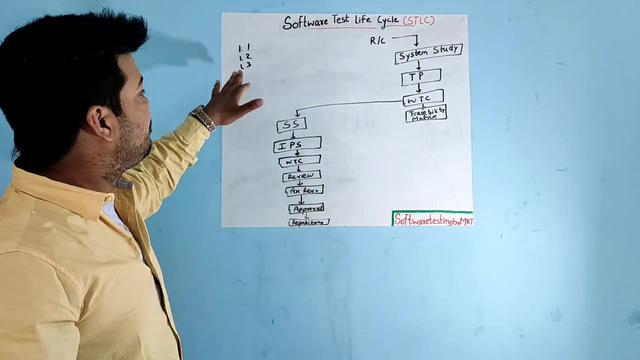 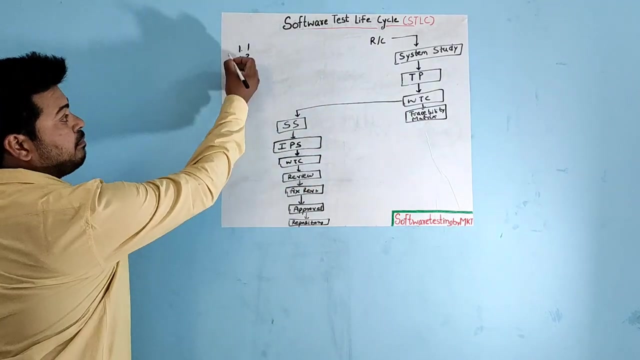 That is nothing but traceability matrix. So we will see the requirement And we will see for each and every requirement There is a particular test cases there or not. If any of the requirement Has not got any particular test cases, Then we can go and mark that requirement. 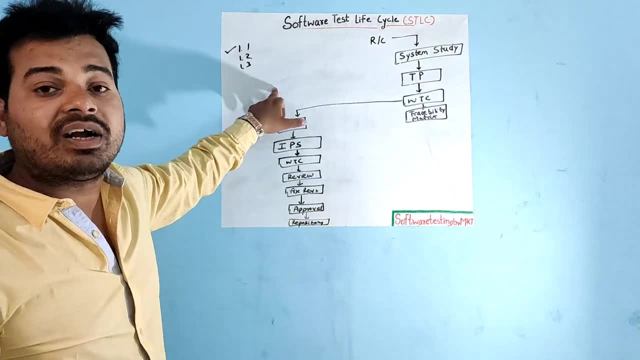 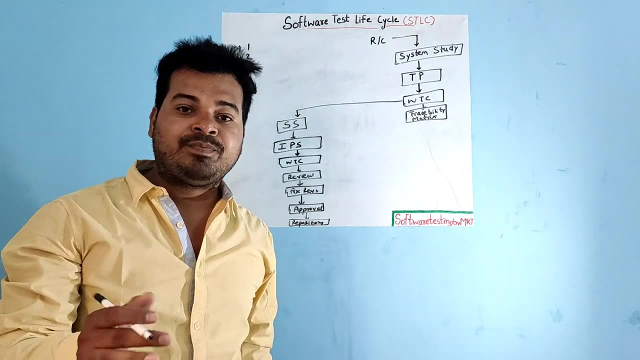 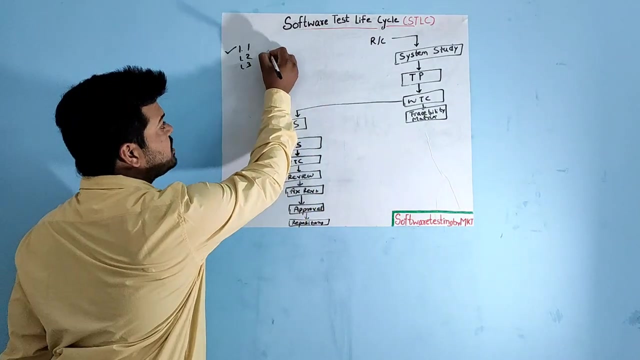 And if other requirements have got at least one test cases in it, We can unmark it. So this is called as traceability matrix. Now there are three types of traceability matrix we have. The first type of traceability matrix Is called as forward traceability matrix. 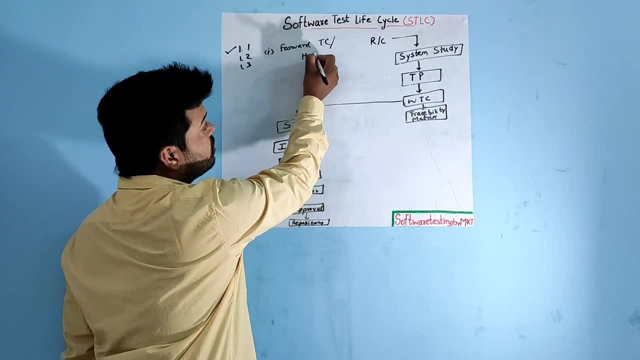 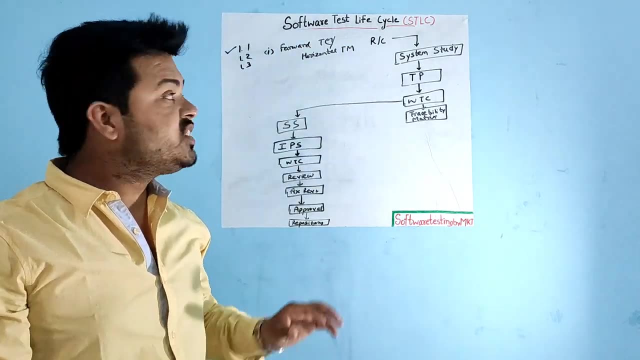 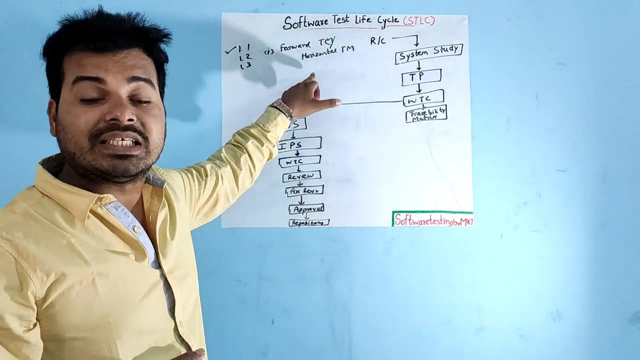 Which is also called as horizontal traceability matrix. Forward traceability matrix is nothing but Here we ensure that Each and every requirement Has got at least one test cases in it or not. Forward traceability matrix is prepared Before our test case execution. 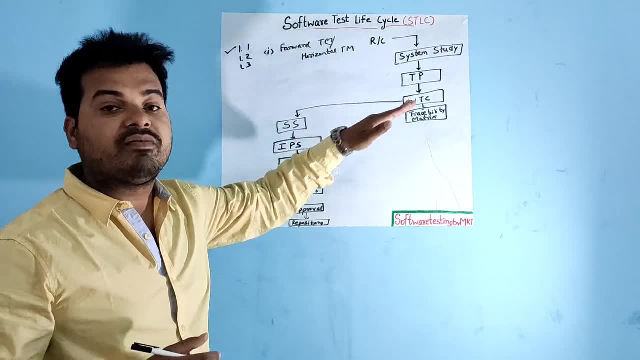 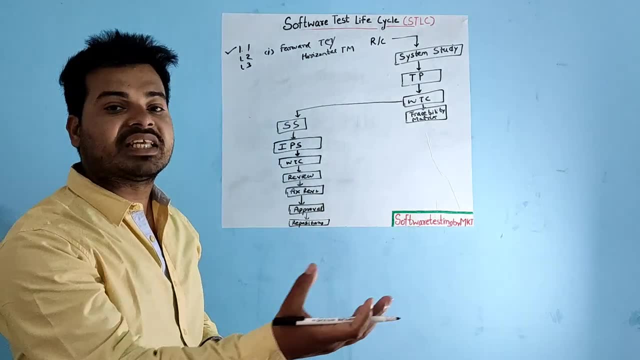 So, once after my test cases is done, We will prepare the traceability matrix. Once after traceability matrix is prepared, Finally, we are going to do the test case execution. This is what happened in forward traceability matrix, Which is also called as horizontal traceability matrix. 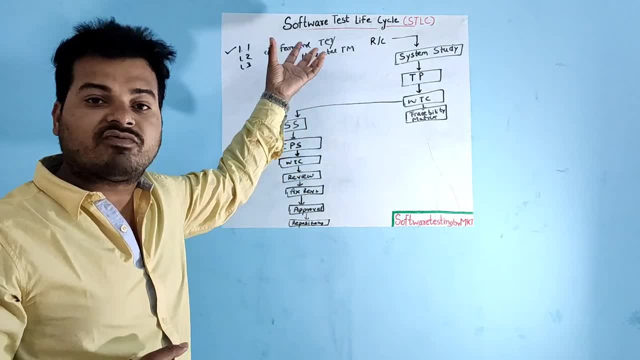 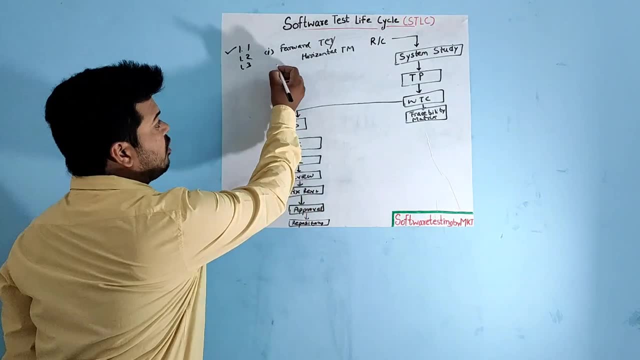 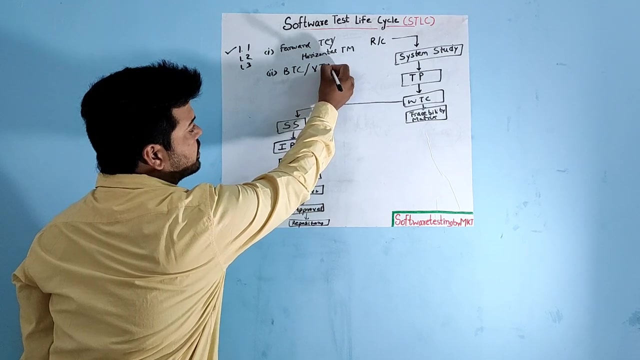 While doing horizontal traceability matrix Or forward traceability matrix, Here we ensure that Are we building product right? The second type of traceability matrix Is called as backward traceability matrix Or vertical traceability matrix. In my backward traceability matrix: 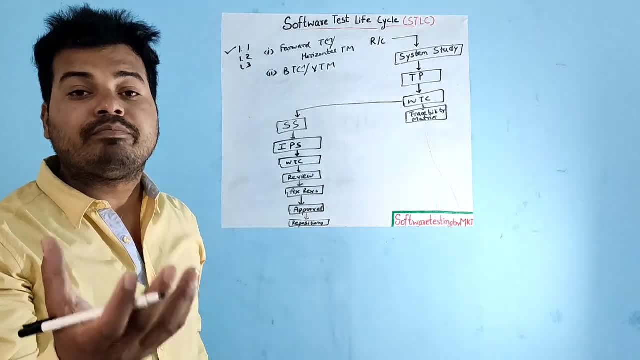 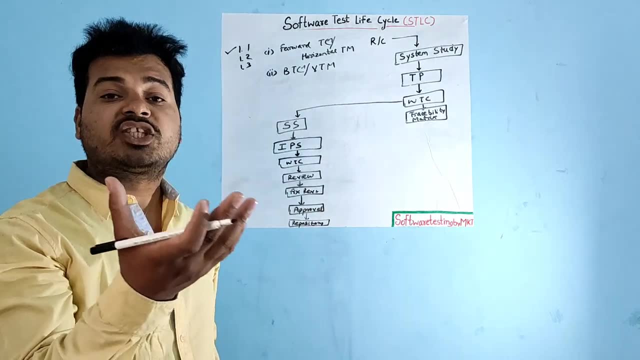 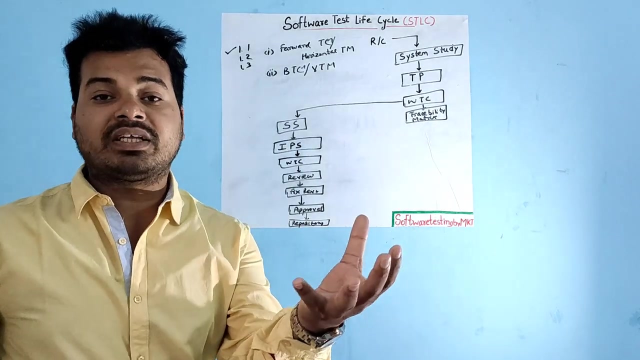 Here we ensure that. Here we map the test cases. Here we map the test cases to the requirement. Here we ensure that The scope of the requirement is not changing, The scope of the development is not changing, Whatever the requirement was given by the customer. 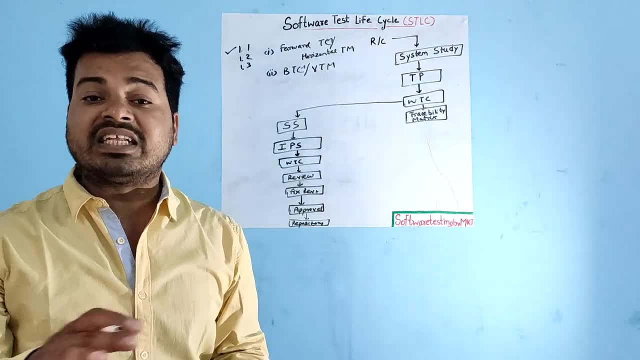 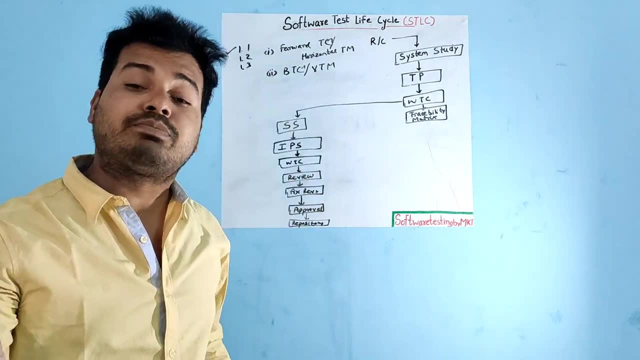 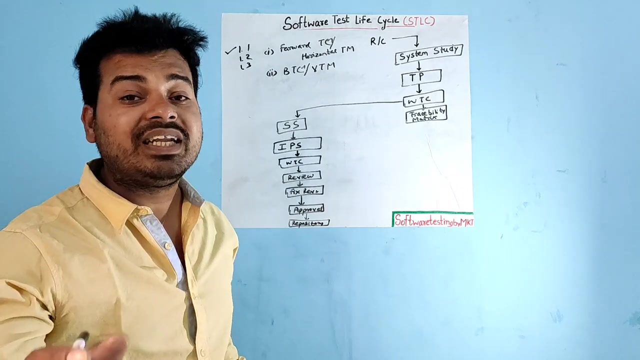 Same thing developer is implementing. Nothing is changed In backward traceability matrix. We ensure all these things And backward traceability matrix Is prepared Once after test execution is done. And, most important here, we ensure that Are we building right product. 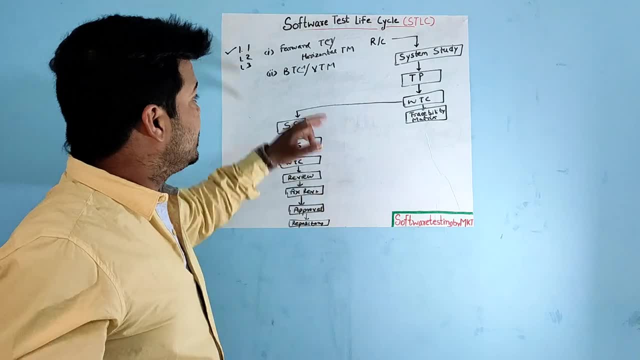 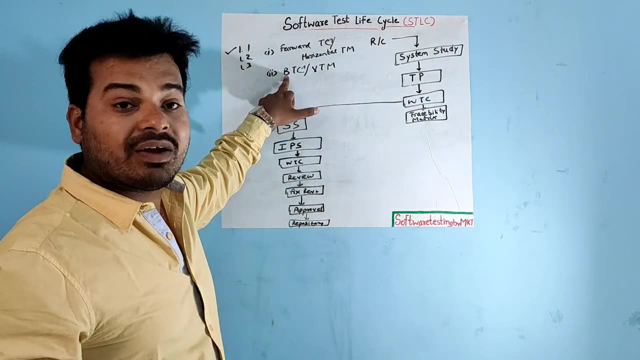 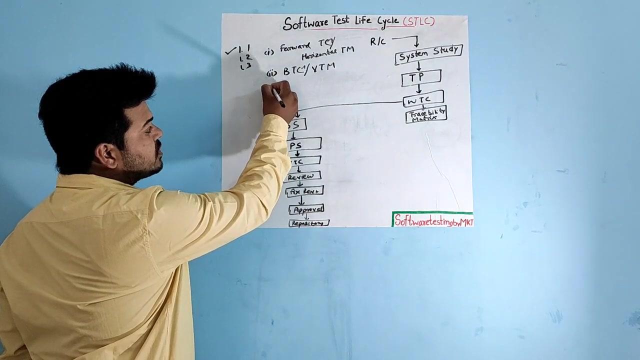 So the main thing which you need to remember is: Forward traceability matrix is prepared Before my test case execution, And backward traceability matrix is prepared After my test case execution. And the third type of traceability matrix Is called as bidirectional traceability matrix. 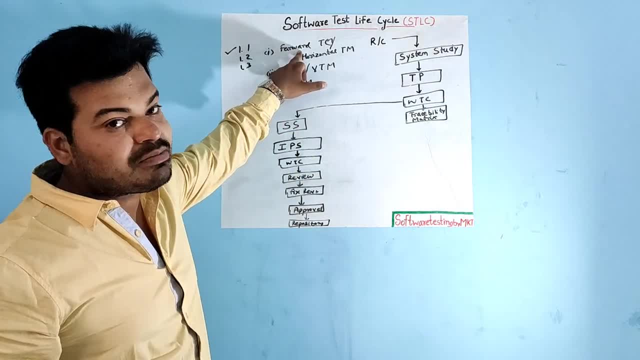 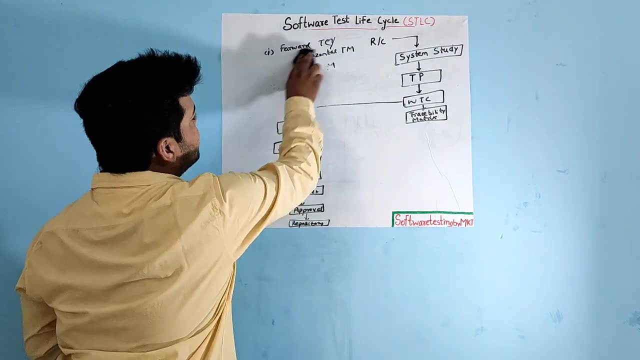 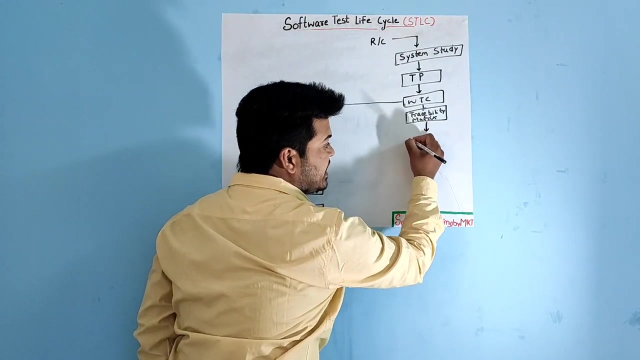 It is a combination of both forward traceability matrix And my backward traceability matrix. So once after my traceability matrix is done, As I told you, Once after my traceability matrix is done, We will do test case execution, We will do execution. 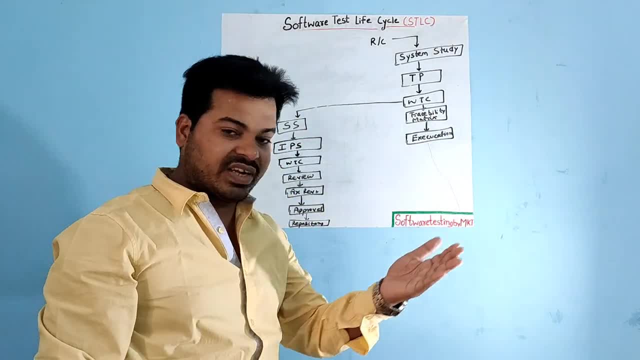 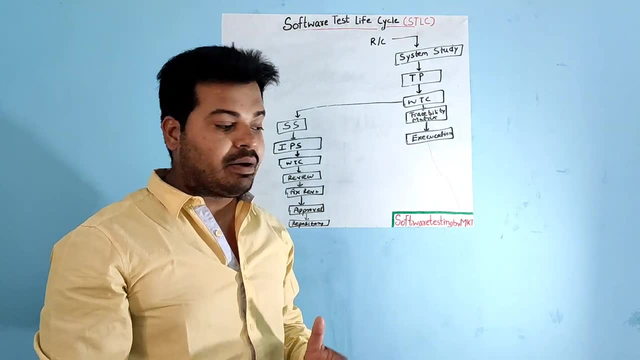 Test case execution is nothing, but You will be having a set of test cases with you And you will be having your application. By looking into the test cases, You will test the application And mark the test cases as pass or fail. So that is nothing but test case execution. 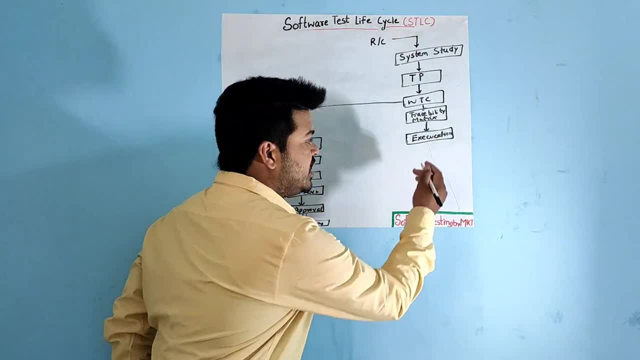 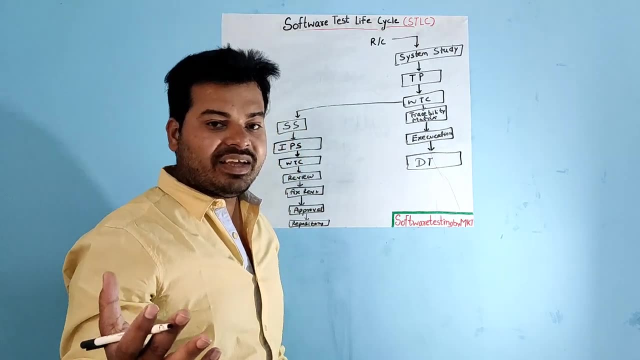 Once after my test execution is done, The next stage of my STLC Is called as defect tracking. Now, what is defect tracking Link is there in the description. Please check it out. I have explained each and everything. If the feature and functionality 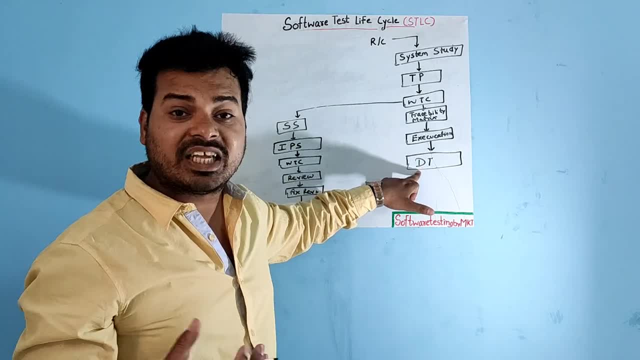 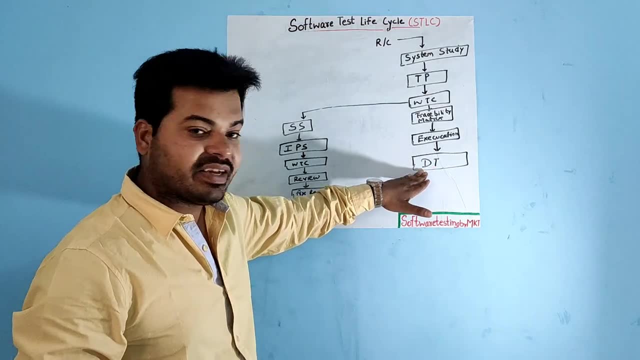 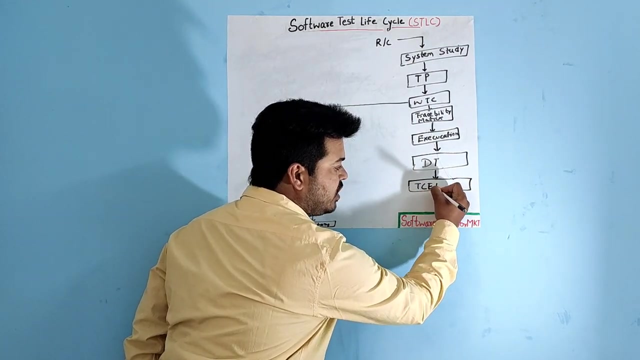 Is not working according to the customer's requirement, Then Qubay or our testers Will raise the defect, Which is nothing but defect tracking. Once after defect tracking is done, The next stage of STLC is called as Test case execution report. 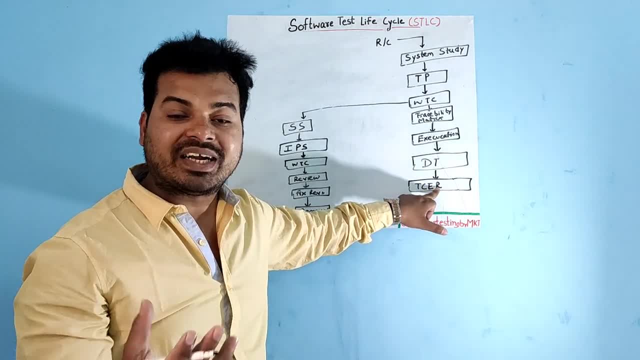 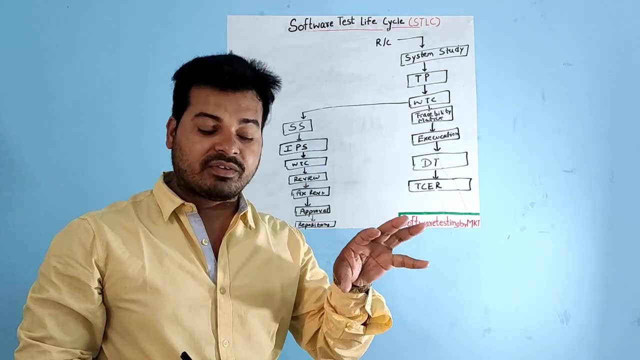 This is the report Which will be prepared by our test lead, In which he will prepare the report Telling that Which test engineers was involved in Which particular module testing And how many bugs we have found out. How many test cases are in the application. 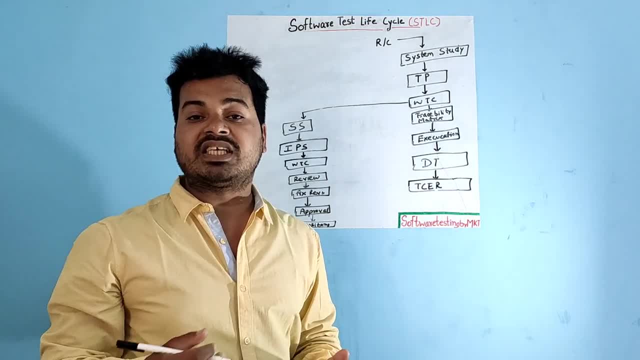 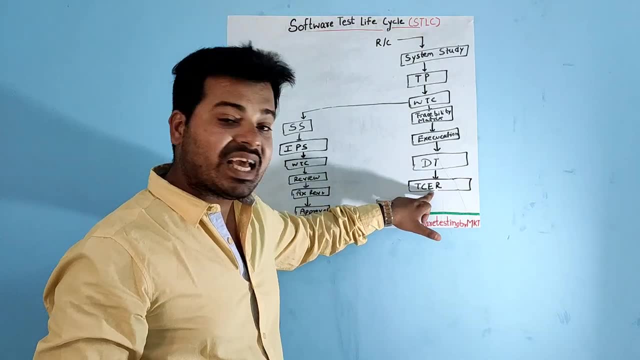 How many test cases are in the past status? How many test cases are failed? What is the past test case percentage? All the report- you will get it in Test case execution report And the final stage of my STLC Is called as retrospective meeting. 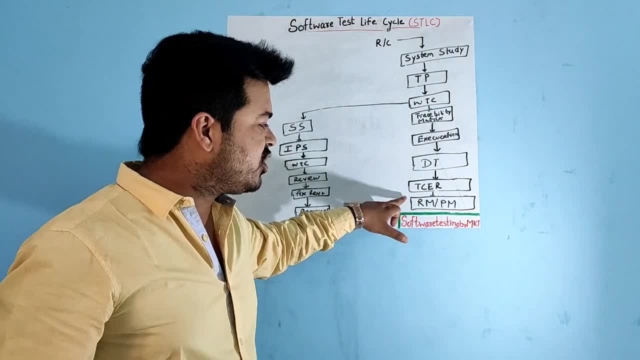 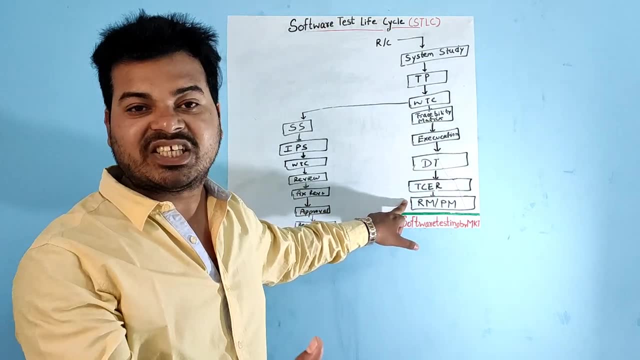 Post-mortem meeting. So retrospective meeting Or post-mortem meeting. It is a meeting conducted by my test manager, Where he will invite all the test engineers Who were involved in this particular relay And he will mainly discuss What went well. 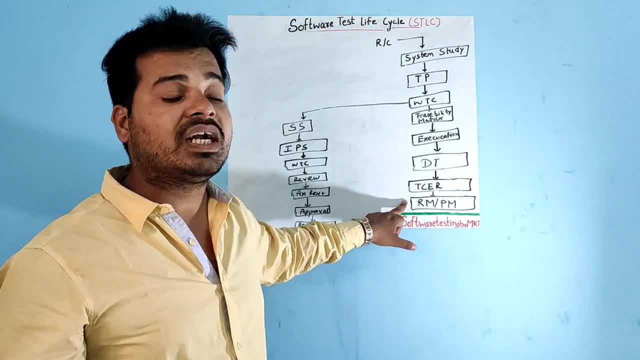 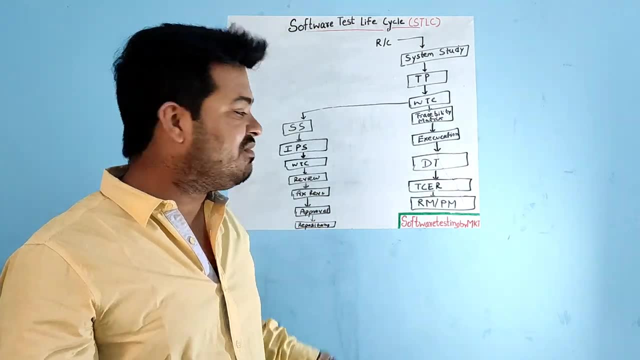 What didn't go well, What are the mistakes we have done, Whatever the achievements we have achieved, How we can improve the process. These and all things he will discuss in the post-mortem meeting. So this is The various stages of STLC. 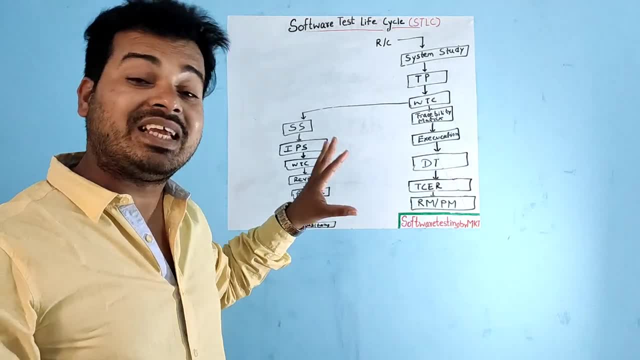 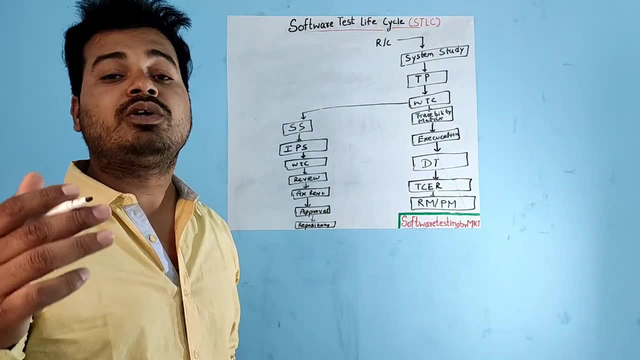 I have tried to explain in a very easy language. If you have any question related to this video, Please ask me in the comment section. If you want to read, If you want to reach to me out personally, I have added my gmail in the link description. 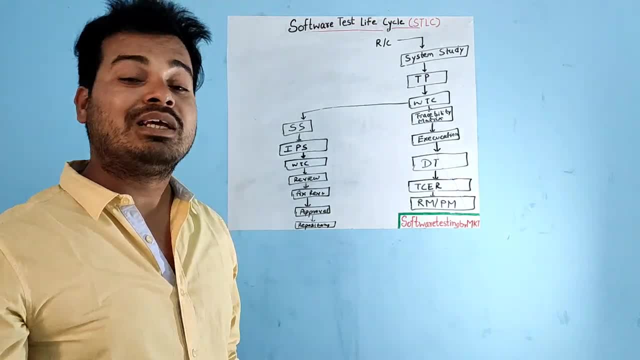 Please check it out. If you think this video was useful to you guys, Please share this video with your needy friends. Like this video. Subscribe to my channel. Software testing by MKT.